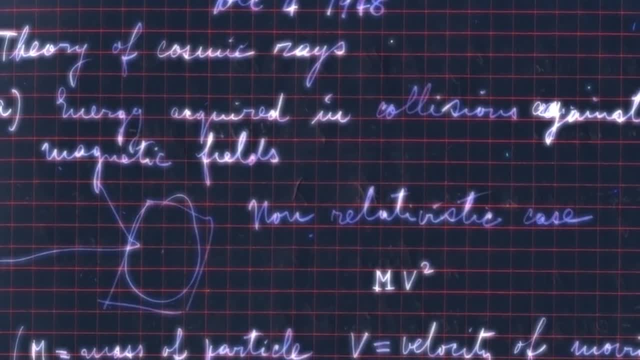 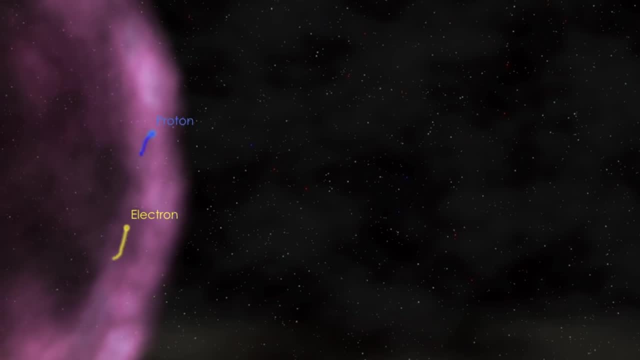 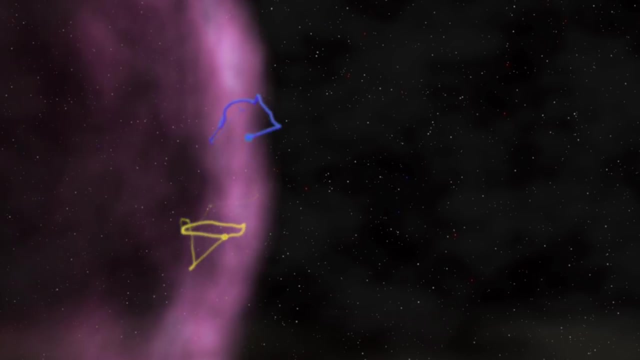 Earth could accelerate cosmic rays. Later studies showed that a variant of his method called Fermi acceleration worked especially well in supernova remnants Confined by a magnetic field, high-energy particles move around randomly. Sometimes they cross the shock wave. With each round trip they gain about 1% of their original energy After dozens to 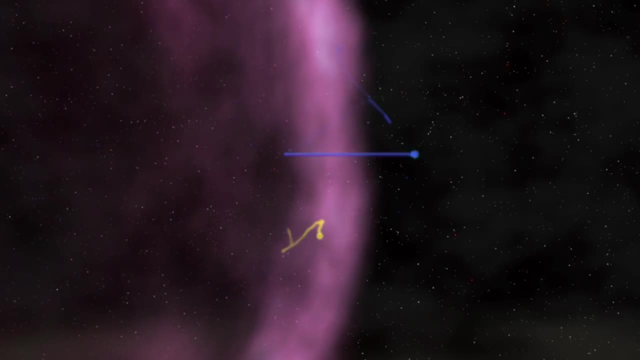 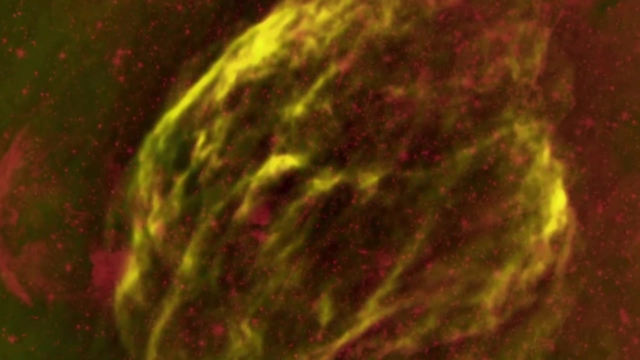 hundreds of crossings, the particle is moving near the speed of light and is finally able to escape. If the supernova remnant resides near a dense molecule, the particle is able to escape Some of the particles that can escape through the rectangular cloud. some of those escaping 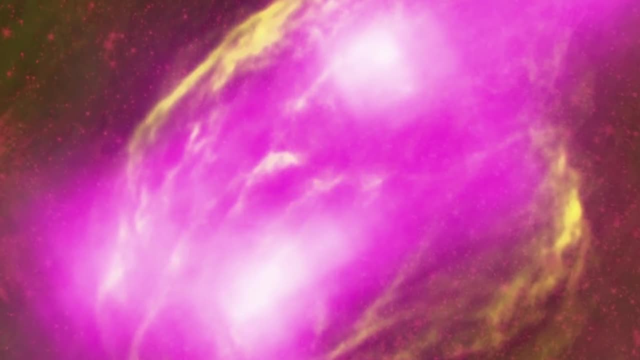 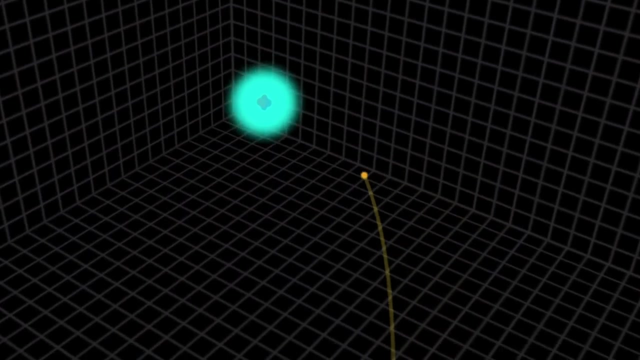 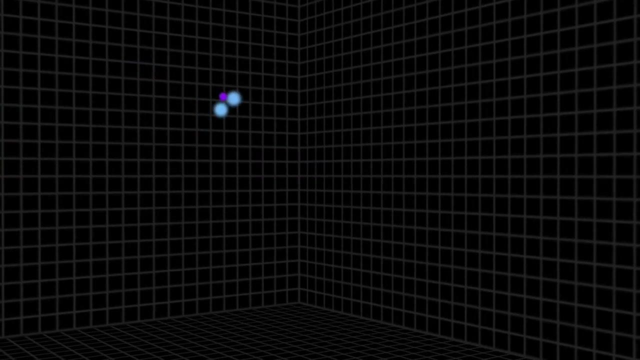 cosmic rays may strike the gas and produce gamma rays, But electrons and protons make gamma rays in different ways. Cosmic ray electrons do so when they're deflected by passing near the nucleus of an atom. Accelerated protons may collide with an ordinary proton and produce a 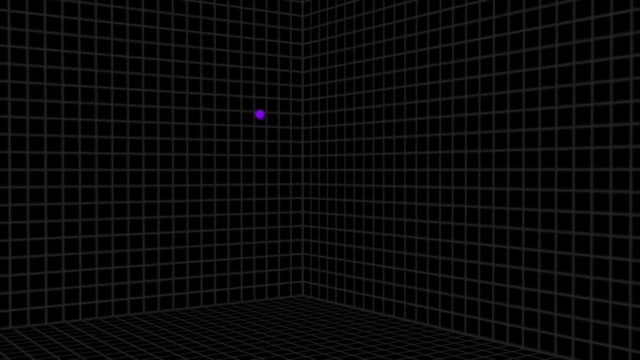 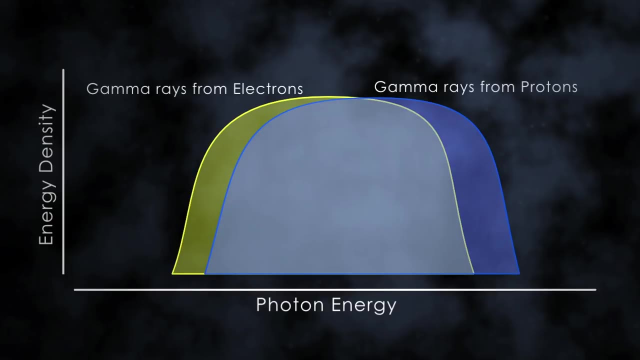 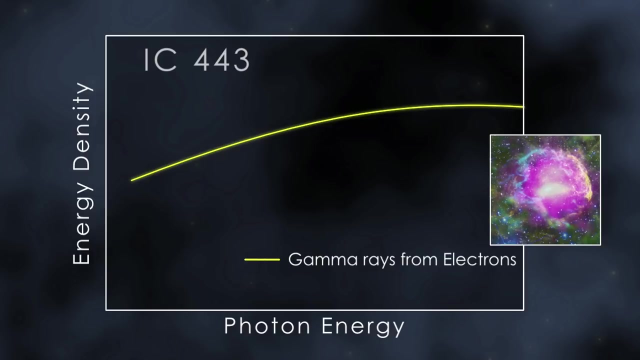 short-lived particle called a neutral pion. These pions quickly decay into a pair of gamma lights. At their brightest, both types of emission look very similar. Only with sensitive measurements at lower gamma-ray energies can scientists determine which process is responsible. Now Fermi observations have done just that. 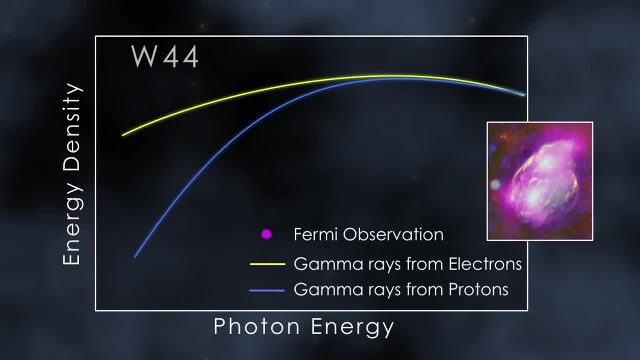 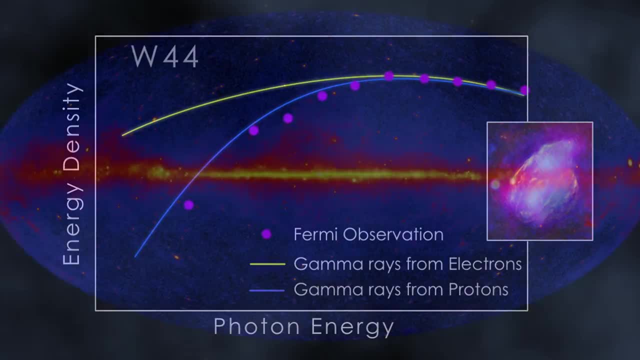 They conclusively show these supernova remnants are accelerating protons. When they strike protons in nearby molecular clouds, they produce pions and ultimately the gamma-ray emission. Fermi sees. NASA's Fermi has detected gamma rays from many more supernova remnants, but the jury. 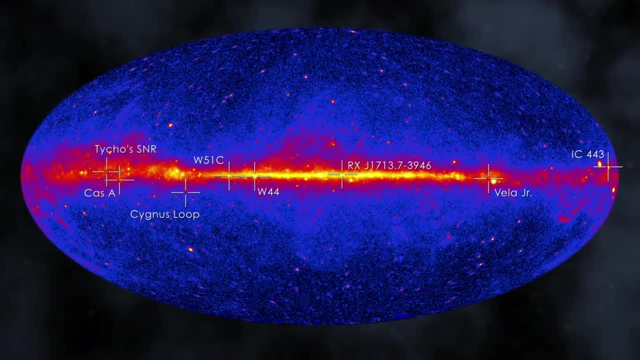 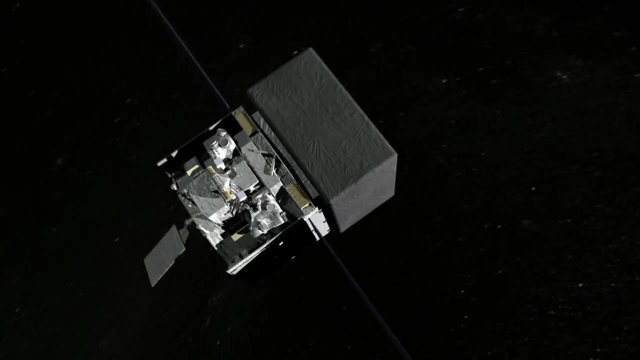 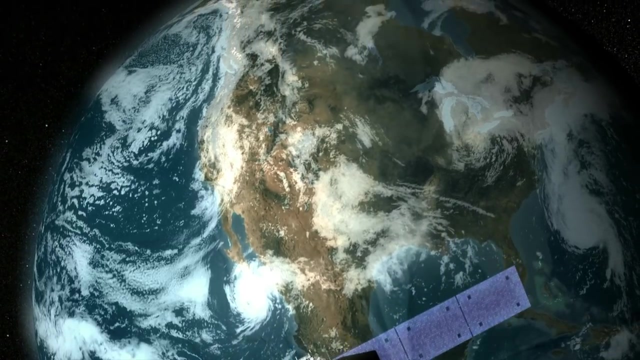 is still out on whether accelerated protons are always responsible and what their maximum energies may be. Nevertheless, the Fermi team has taken a major step, a century after the discovery of cosmic rays, in establishing just where they arise, Something that would satisfy, but certainly not surprise, the original Fermi. Subtitles by the Amaraorg community.